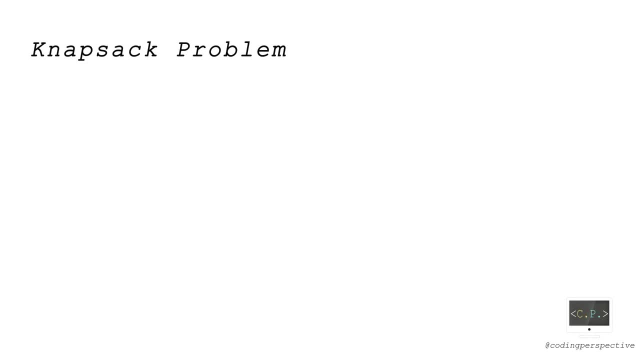 a developer, or if you are a developer, just think about yourself. Let's suppose that there are some projects that you can work on. Depending on the amount of work and difficulties, the time required to complete the project differs, so the money you will gain, For example, you need to. 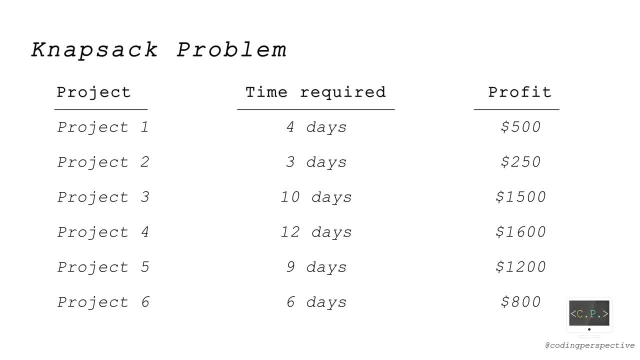 spend 4 days for project 1 to finish it and gain $500, whereas it will take 3 days to finish project 2 and you will gain $250.. Also, let's suppose that each project is due in a month and you cannot. 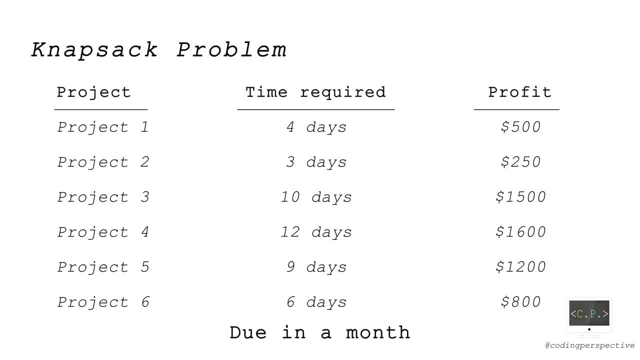 finish all the projects in this time. You need to complete only some of them so that you will gain as much as you can. This problem is called a knapsack problem. If you're allowed to do same projects more than once, then it's an unbounded knapsack problem. Otherwise, 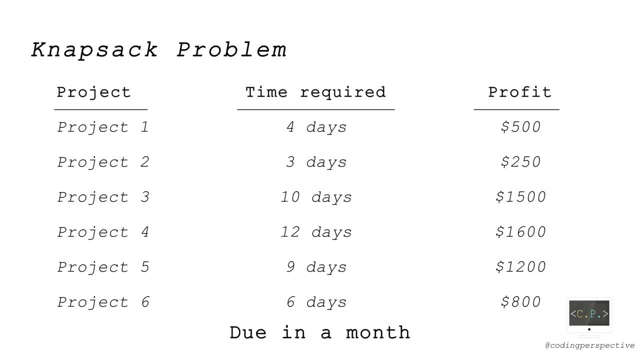 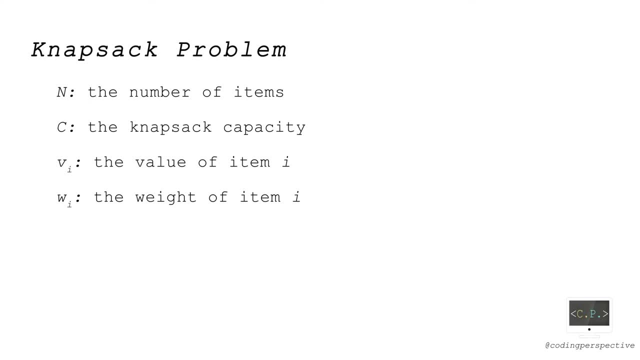 it's called binary or 0-1 knapsack problem, where you choose either to do project or not. To formulate the problem, let me introduce you some notation. First, let N be the number of items, or like the number of projects that you can work on in our example. Then let C be the 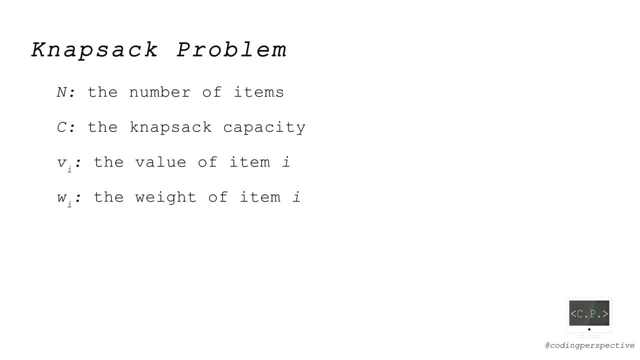 the knapsack capacity a month or 30 days in our case. Also, let the i denote the value of item i, or, like, the amount of money you will gain from project i. Lastly, wi denotes the weight of item i, which correspond to the amount of time required. 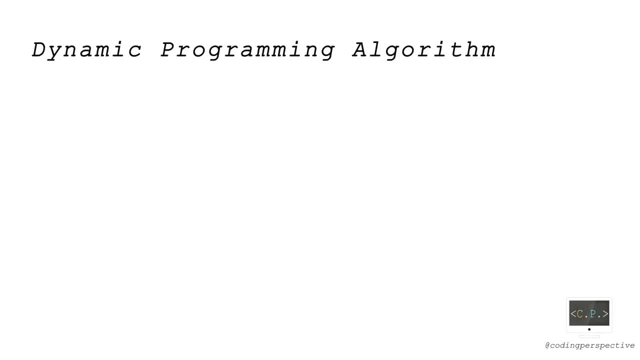 to complete project i in the example. Now we are ready to formulate the problem and solve it by using dynamic programming. Before showing you how to do it, it's worth mentioning that we can solve this problem by using mathematical optimization as well. To learn how to do it in Python, please click the link above. 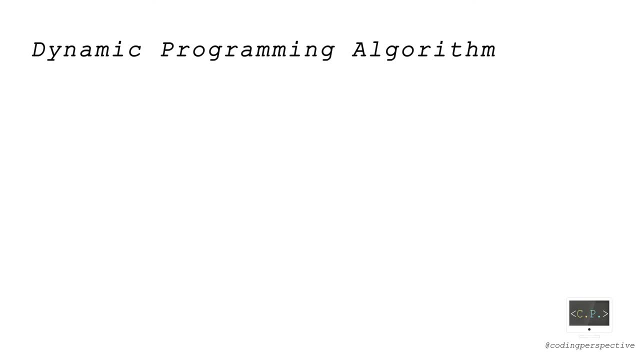 Here I will focus on how to solve the binary knapsack problem instead of the unbounded one. Now let's develop our dynamic programming algorithm to solve it. First, we construct the value function mic for each item i and capacity c. mic represents the maximum value that can be obtained. 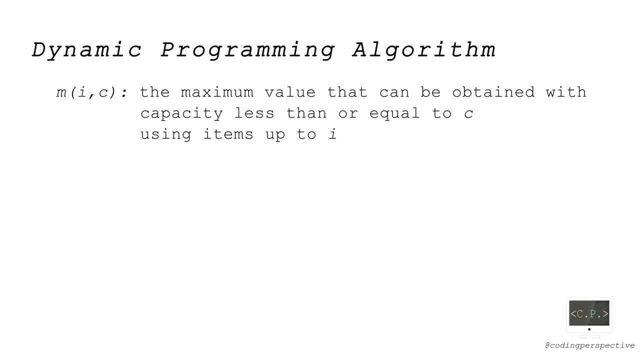 with capacity less than or equal to c using items up to and down. Note that the solution to the problem can be obtained by computing m, capital, N, capital C as its maximum value with capacity is less than or equal to c using all items. In the first step, we initialize the value functions. 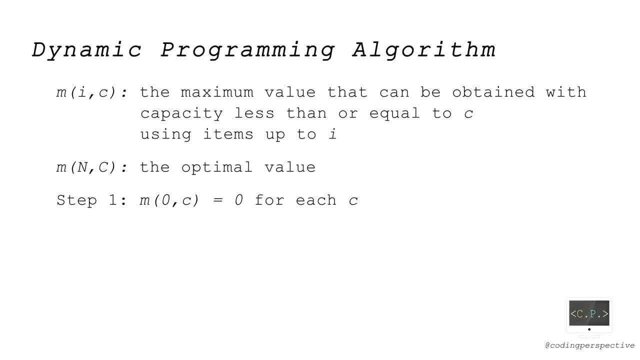 m0c equals to 0 for each c because no item is included. Then in the second step, using a nested loop, we iteratively update mic as follows: To compute m0c, we have only two options for item i. If we don't include item i and leave it out, 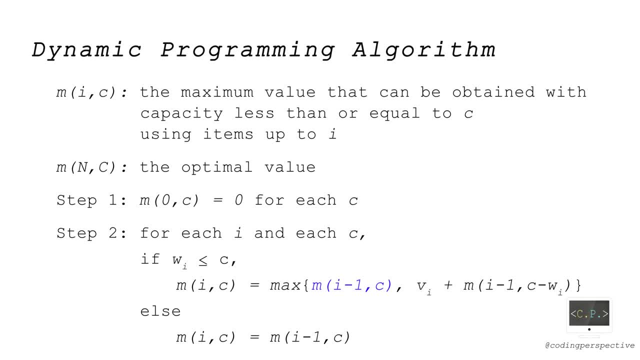 then the best we can do with items up to i minus one and capacity c is m i minus one c. If we include item i then we gain v i but we need w i weight in return. So the best we can do with the remaining items up to i minus one. 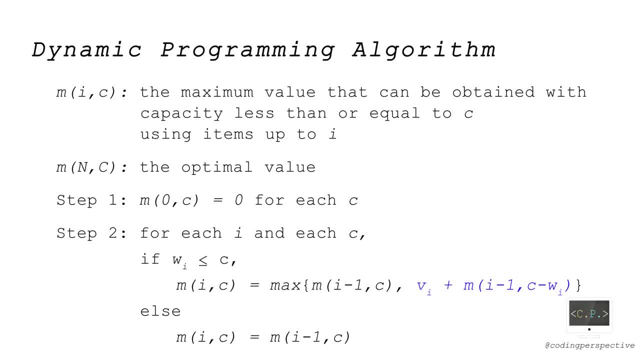 and capacity: c minus w i is m i minus one, c minus w i. Thus we get v i plus m i minus one and c minus w i, if we can include item i. Note that we can include item i only if w i is less than or equal to c. 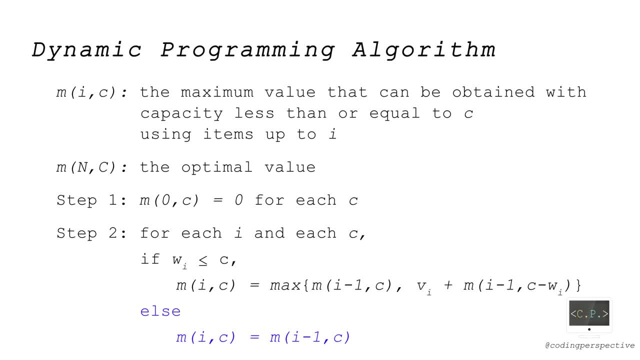 Otherwise we cannot include it, so that m i c is equal to m? i minus one c. Hence we can compute m i c in this way for any item i and capacity c. It's clear from the nested loop that m i c equals m? i minus one c. 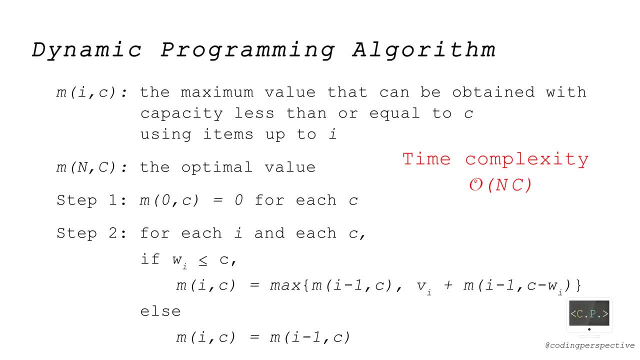 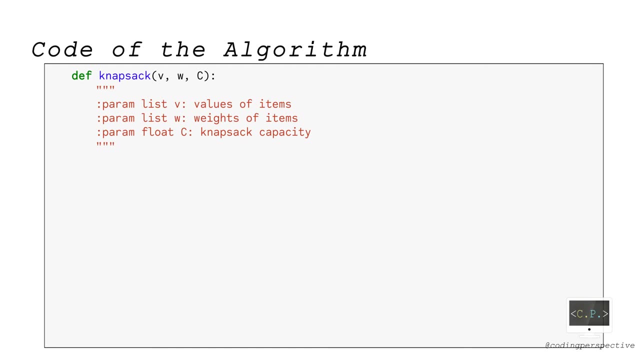 it looked that the time complexity of this algorithm is order of capital N times capital C And the speed complexity is also order of capital N times capital C, from the size of the value functions. Now let's code this algorithm in Python by writing a function called knapsack. 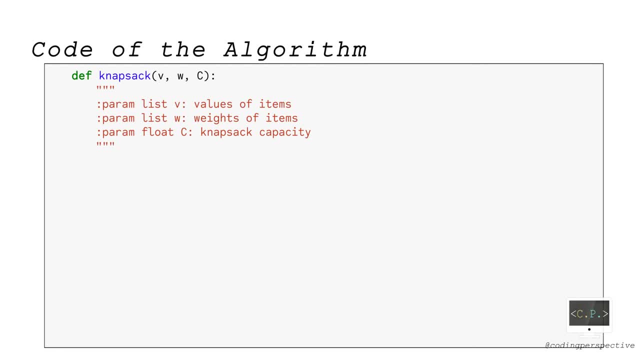 The inputs of this function are the values and weights of the items as list and capacity as a full-order. First we compute the number of items, capital N. Then, in the first step, we initialize the value functions m0c to 0 for each c. 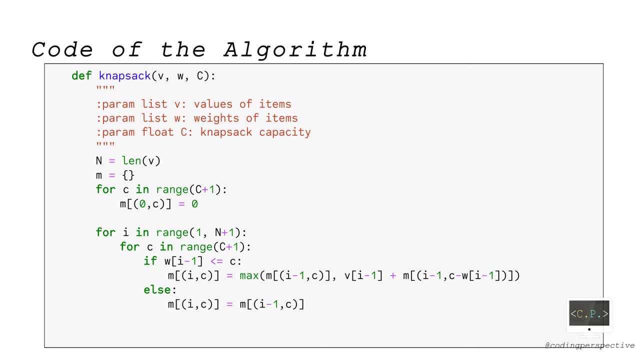 In the second step we have a nested loop. In the outer loop, we iterate over each i from 1 to capital N, whereas we iterate over each c in the inner loop. We update the value function mic in this nested loop. Lastly, we return mNC the maximum value obtained with capital C as an output.